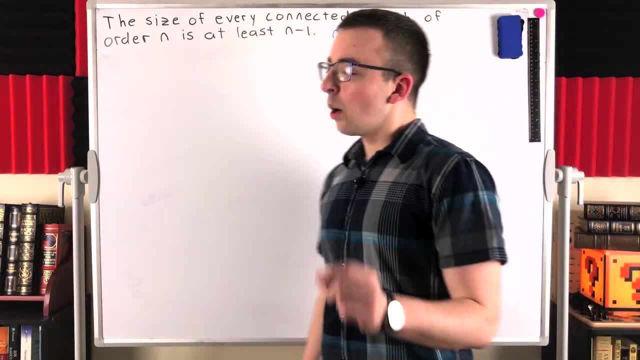 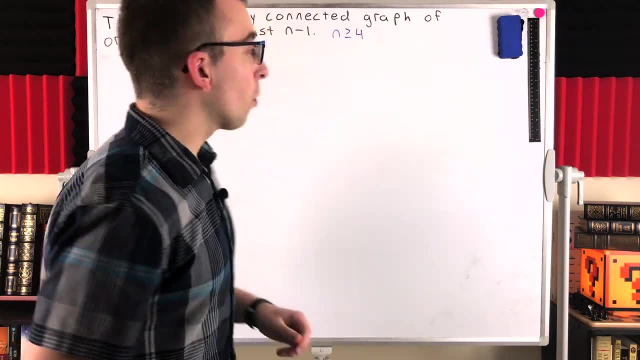 Now, among all such counter examples to our claim, we're going to pick out a minimum counter example, which is why this is called a proof by minimum counter example. In particular, we're going to minimize the order. So, among all such counter examples to our claim, let's pick out a graph g. 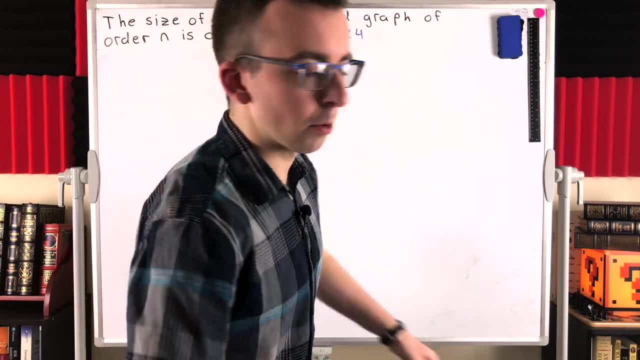 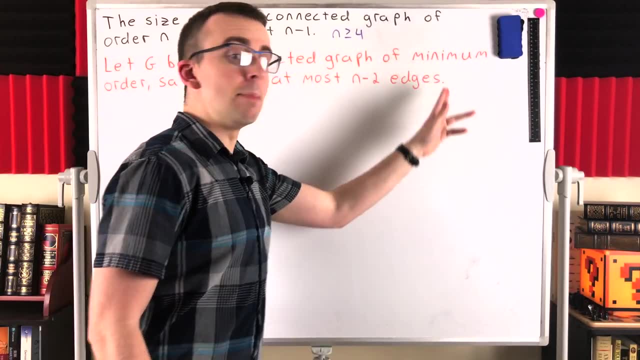 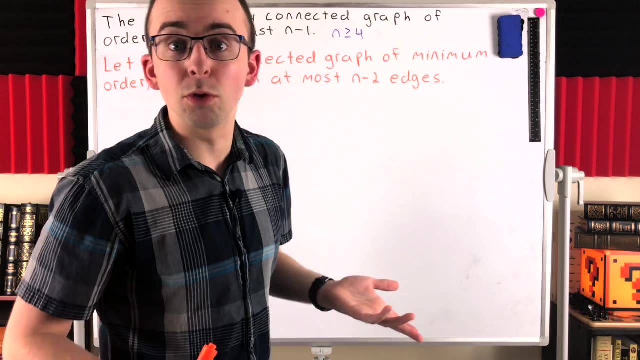 that has the fewest number of vertices. among all those counter examples, I'll write that now. So, among all counter examples to our claim, we're going to say that g is a minimum, a counter example of g. There might be multiple counter examples with the same order. We're just going to say g is one of. 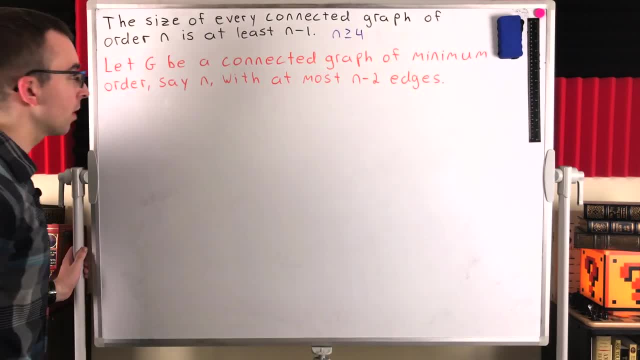 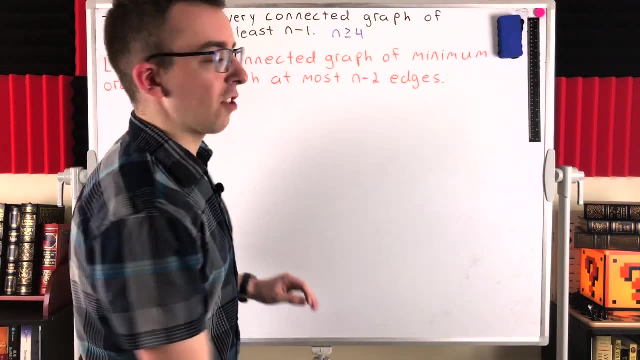 them. In order for it to be a counter example, it's got to be a connected graph. We're going to call its minimum order n and again, for it to be a counter example, it's got to have at most n minus two edges. So that's strictly less than n minus one edges. Now the idea of this proof by minimum. 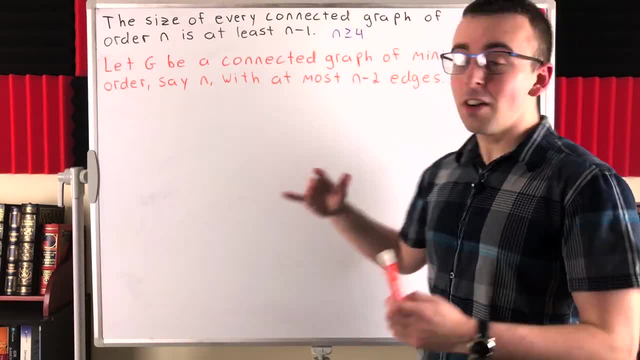 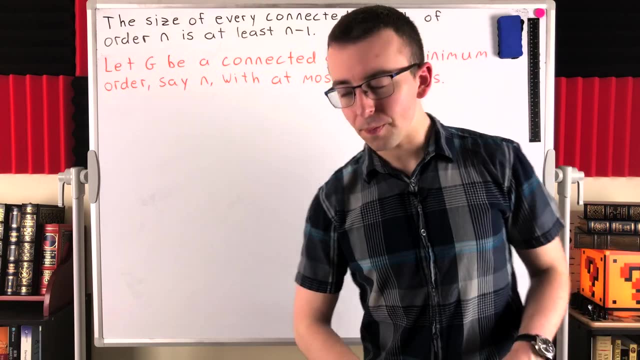 counter example is. we want to show that this is, in fact, not a minimum counter example, which is going to produce a contradiction, thus showing that our claim is not a minimum counter example Actually must be true. So to find a counter example that is more minimal than this one, you 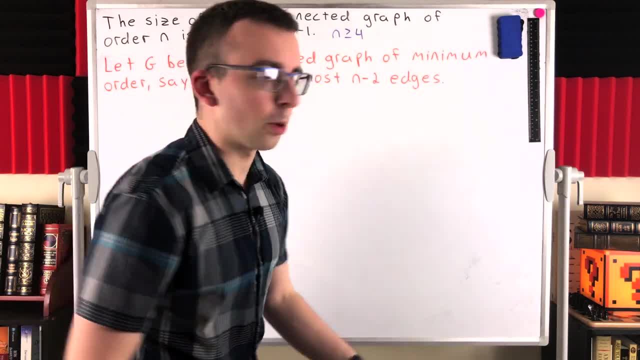 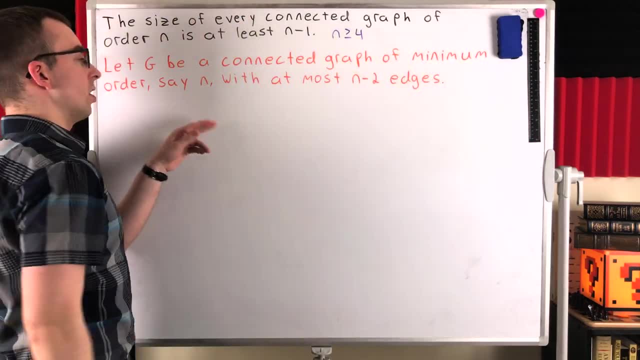 might think we'll have to delete a vertex from g. Then we can have a counter example that has fewer vertices from g, fewer vertices than g. Excuse me contradicting the fact that g is a minimum counter example, But remember, to contradict our claim, a graph has to be connected, So we can't. 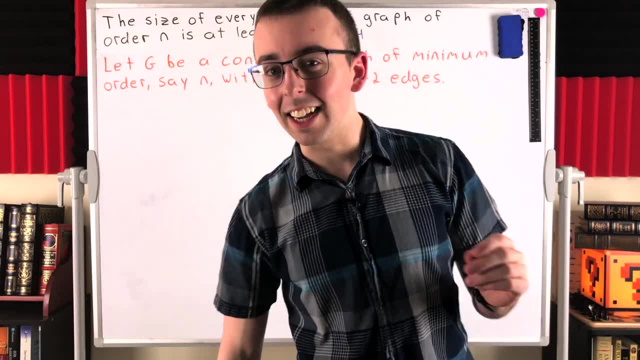 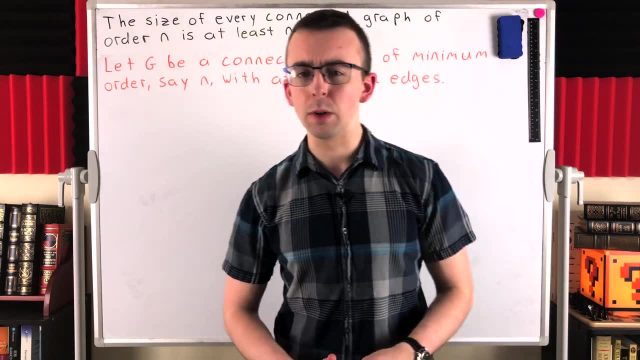 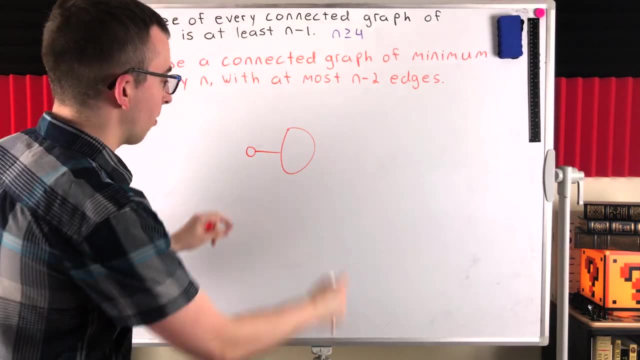 just delete any vertex from g. We don't want to accidentally delete a cut vertex. So what type of vertex is never a cut vertex? Well, that would be an end vertex, a vertex of degree one. You can never disconnect the graph by deleting a vertex of degree one Looks something like that: 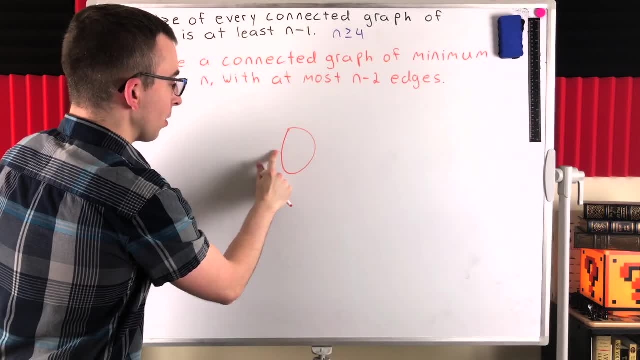 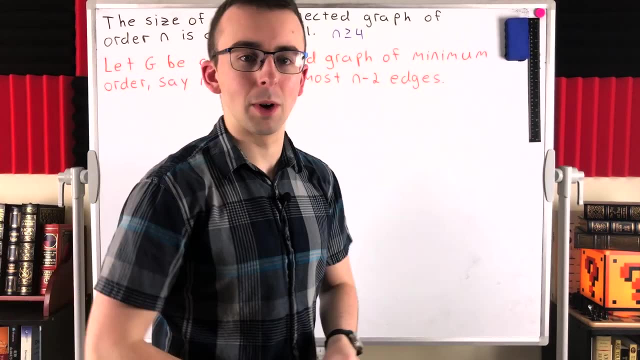 right, You got a graph and here's a vertex of degree one. You'll never disconnect the graph by deleting a vertex of degree one, So we would like it if g had a vertex of degree one so that we could delete it and be sure that the resulting graph was still connected. So then we'll claim: 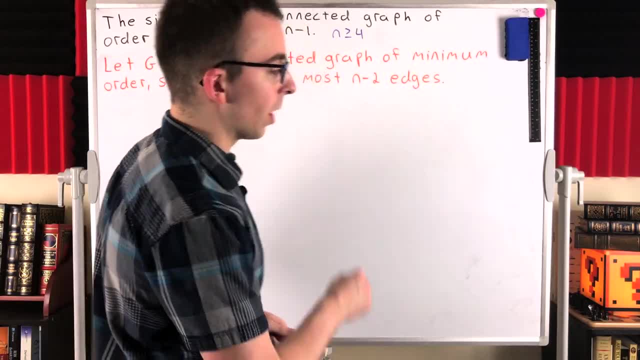 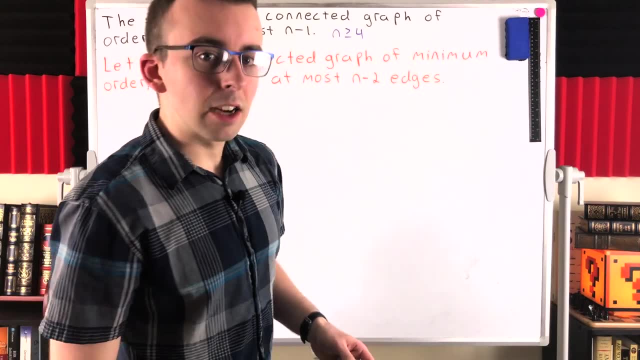 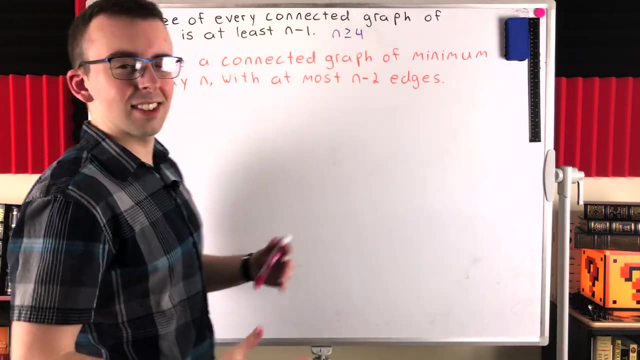 g does have an end vertex, a vertex of degree one. Why must it Well suppose, for the sake of contradiction, that g does not have an end vertex? We also know it doesn't have any isolated vertices, because it's a connected graph. that's non-trivial, since it's got to have at least four. 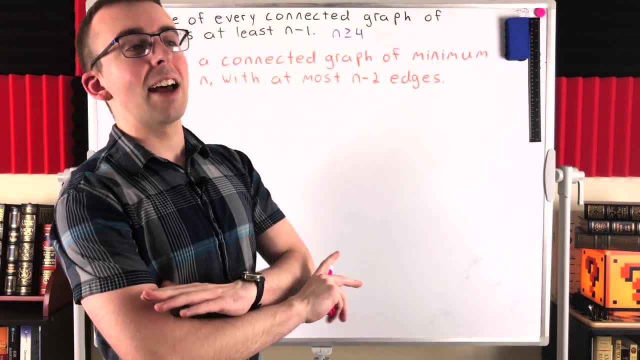 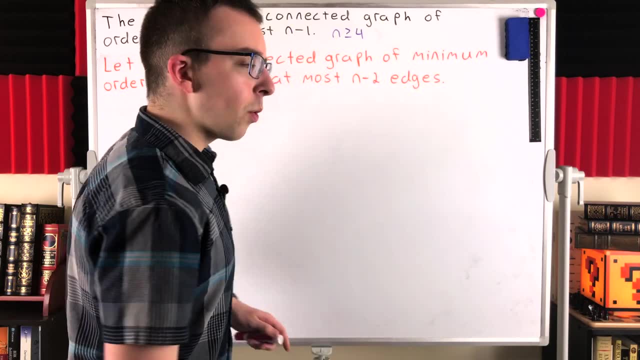 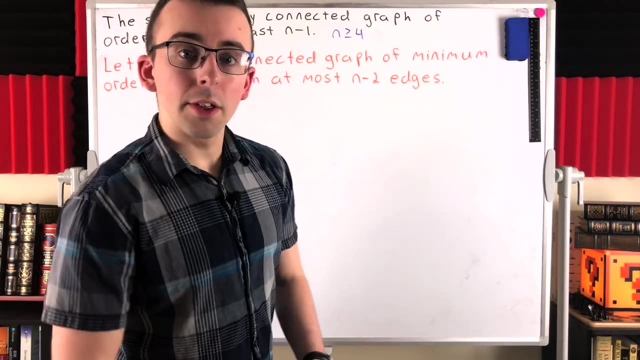 vertices. So it's connected non-trivial, which means it has no isolated vertices of degree zero. We're assuming for the sake of contradiction. it has no vertices of degree one. So every vertex in g must have a degree of at least two. Now what if we add up all the degrees of all the? 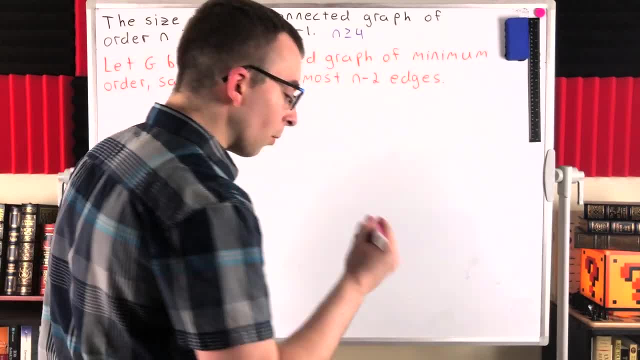 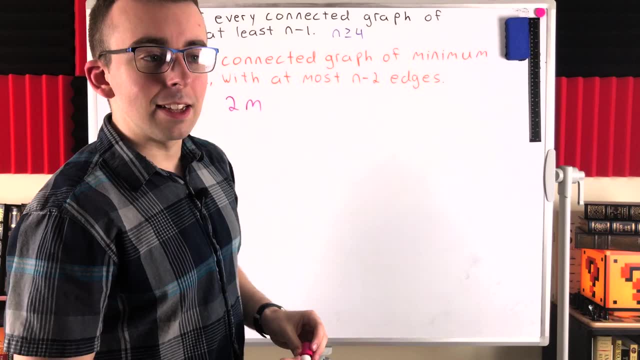 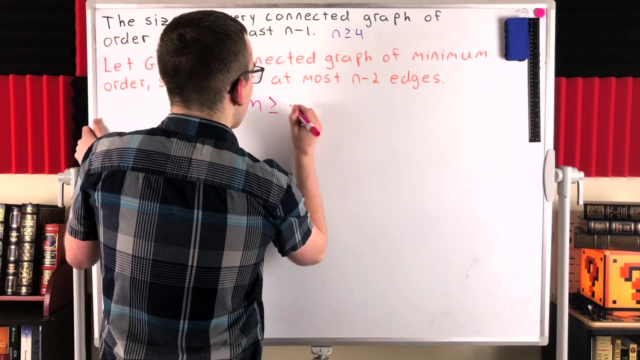 vertices in g. What a squeaky marker. Well, by the first theorem of graph theory, if we add up all of the degrees of the vertices in g, that's equal to two times m, where m is the size of the graph, the number of edges. Since the degree of every vertex is at least two, this has to be greater than or. 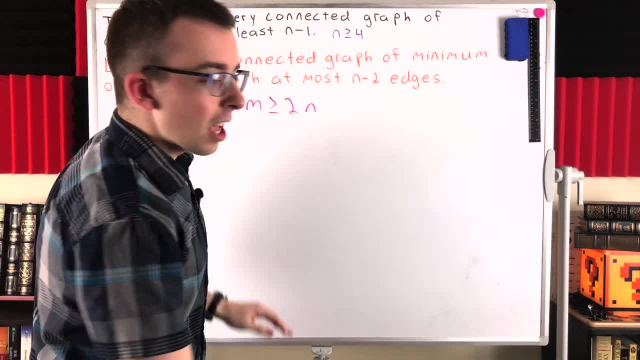 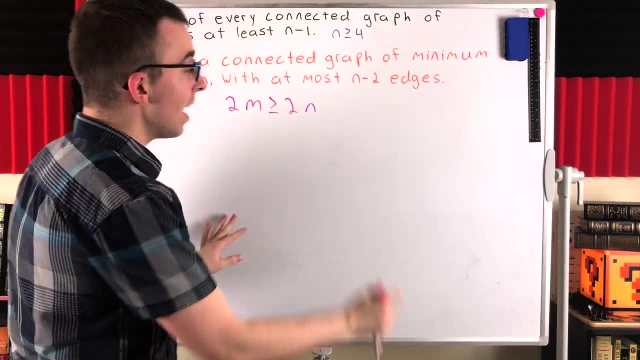 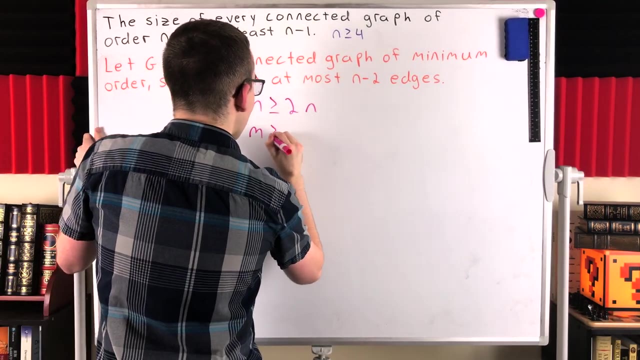 equal to two times n, Two times the number of vertices, because every vertex is going to be two, and so we want to contribute at least two to the degree sum. So two times m, the degree sum has to be greater than or equal to two times n. We can divide both sides of this inequality by two to get that m. 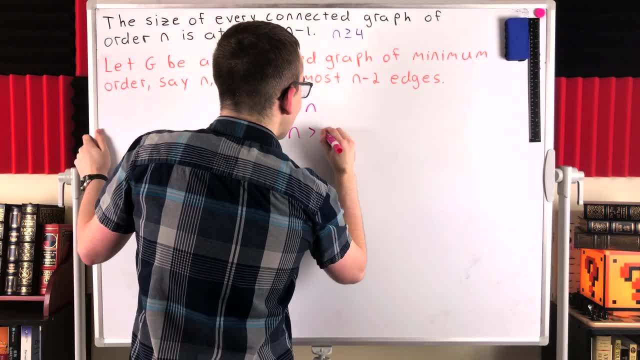 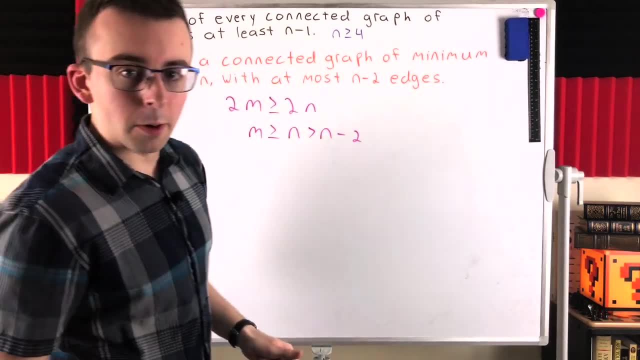 is greater than or equal to n, and notice that n is strictly greater than n minus two. That's a problem, because we assumed that m, the size of our minimum counterexample g, was at most n minus two. Here we see the size: M is greater than n minus three. 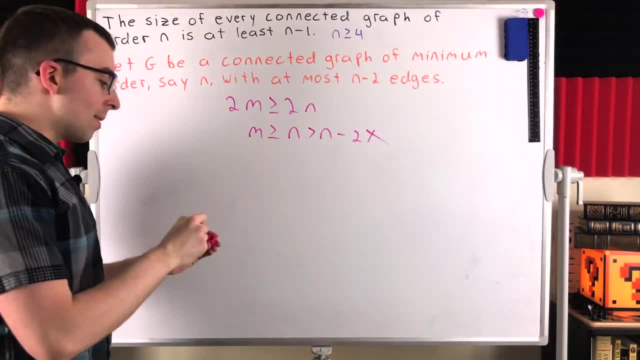 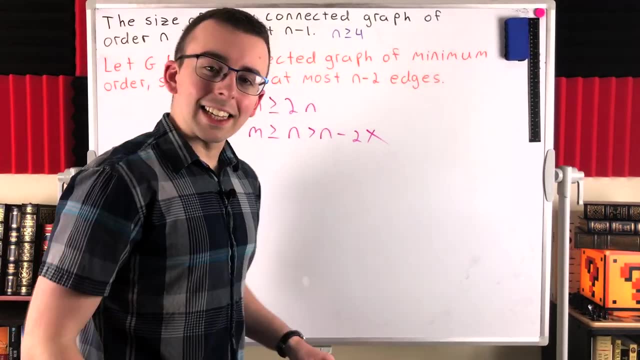 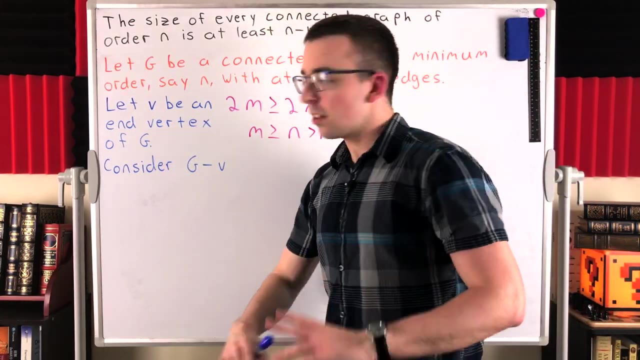 too. So that's a contradiction that can't be so. it must be the case that g does have an end vertex, We'll call that end vertex v and we'll delete it. So let me write that now. So we're saying: let v be an end vertex of g. it's a vertex we proved had to exist in g. it's got to. 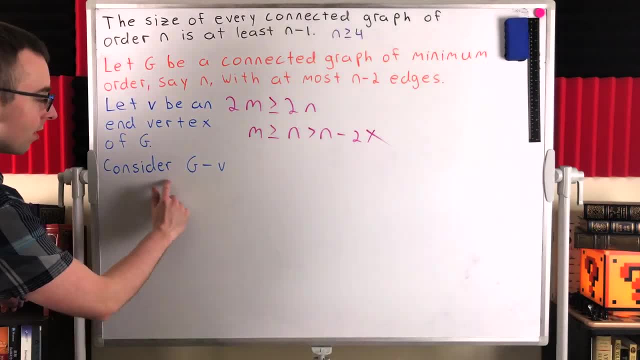 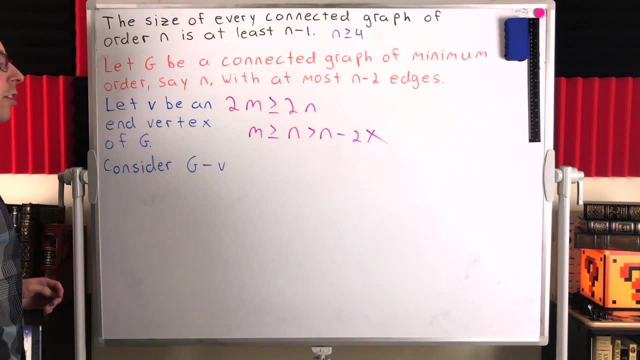 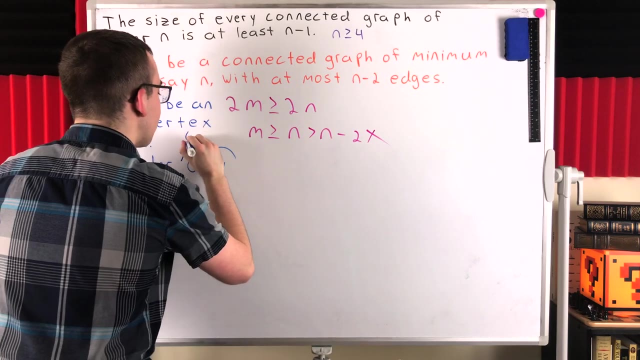 have an end vertex, So let v be an end vertex. and now consider g minus v. We want to show that g minus v is actually a counterexample to our claim that has fewer vertices than g. First thing we want to point out: why did we talk about end vertices so much? Well, g minus v has to be connected because 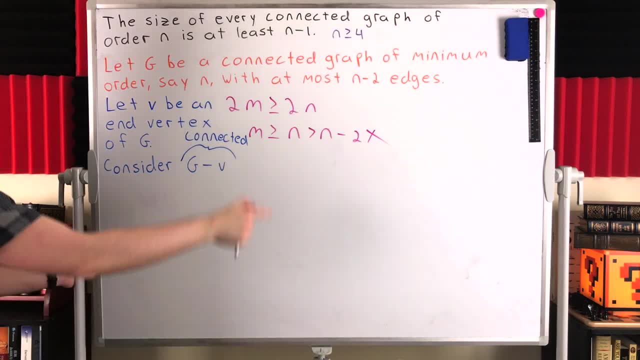 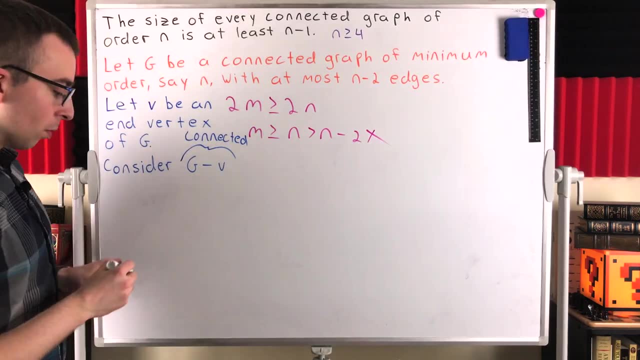 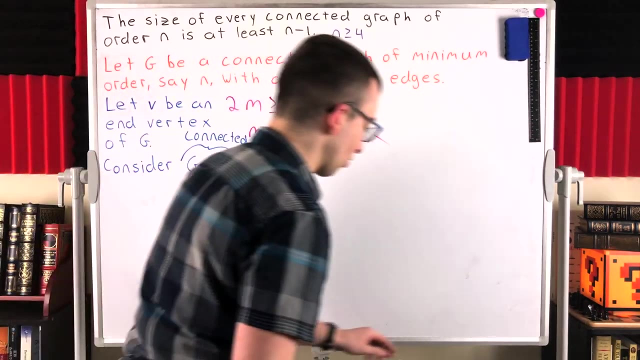 g is connected. Remember that g is a counterexample to our claim, which means it has to be connected, and you can't disconnect a connected graph by deleting an end vertex. So g minus v is connected. all we have left to do, then, is to show that g doesn't satisfy this part of our condition. 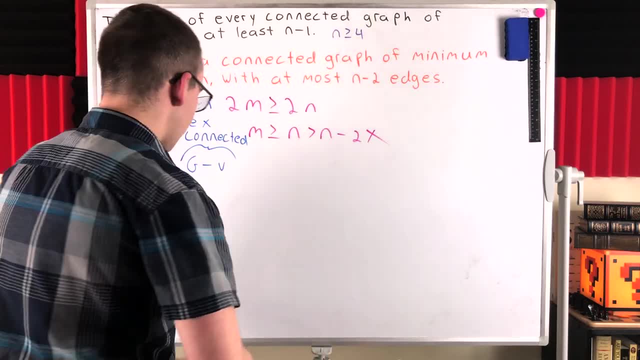 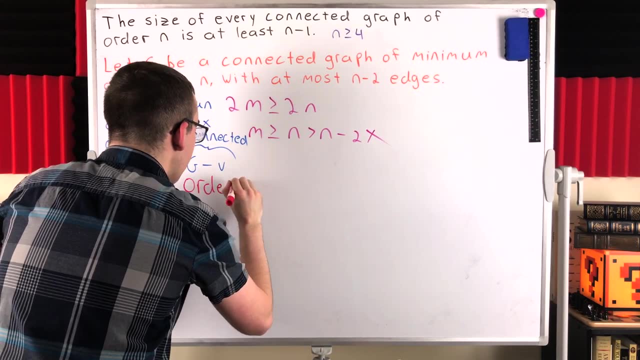 and thus is a counterexample. Let me write in red. So what's the order of g? The order or, excuse me, the order of g minus v. Well, the order of g was n and we deleted one vertex to get to g minus v. 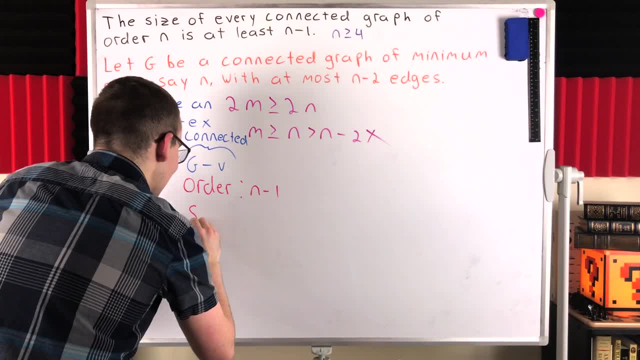 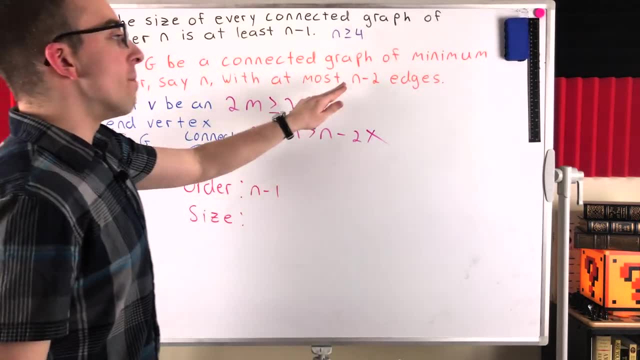 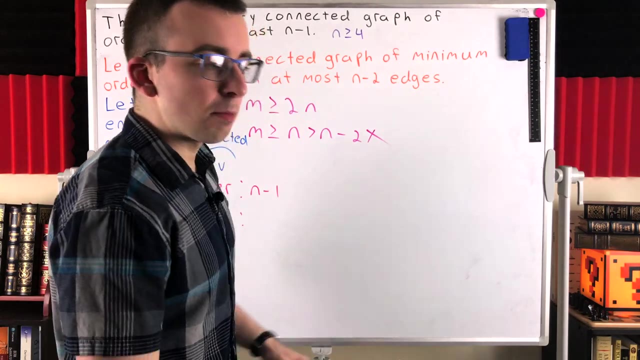 So the order of g minus v is n minus 1.. Now, what is the size of g minus v? Well, the size of g was, at most, n minus 2.. When we delete an end vertex, we're deleting exactly one edge, because an end vertex is incident to exactly one. 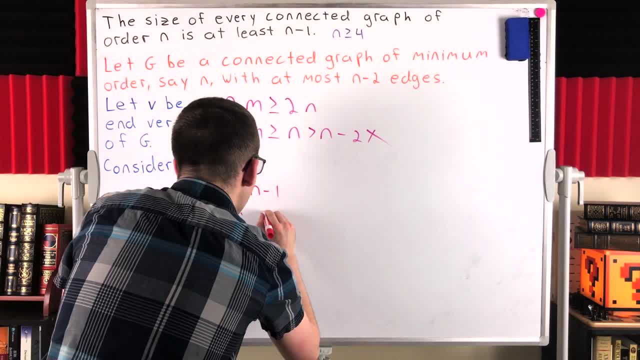 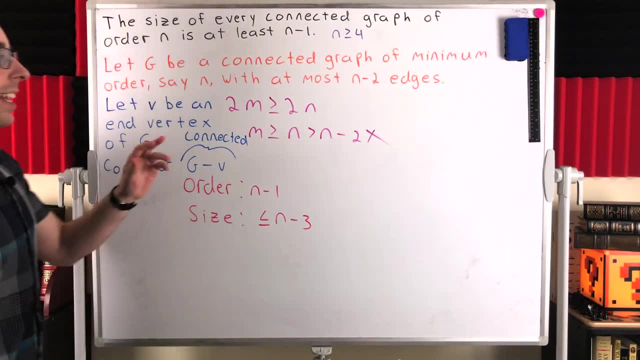 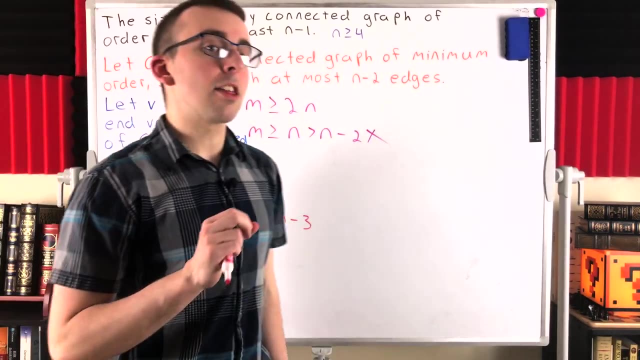 edge. So the size of g minus v will have to be at most so less than or equal to, at most n minus 3.. Again, g had at most n minus 2 edges. we got rid of exactly one. so g minus v has at most n minus. 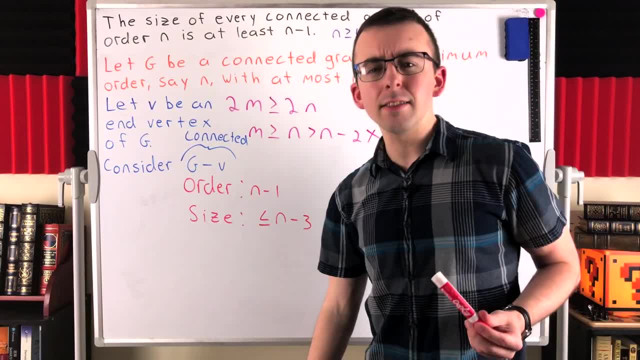 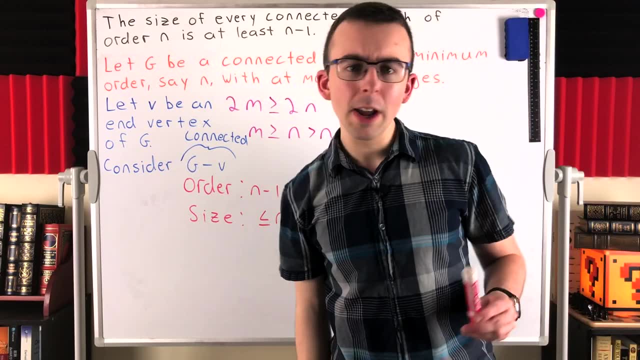 3 edges, And so that shows that g minus v is a counterexample to our claim. Remember, our claim was that every connected graph has to have at least one less edge than it has vertices, But we see that g minus v is a connected graph that has 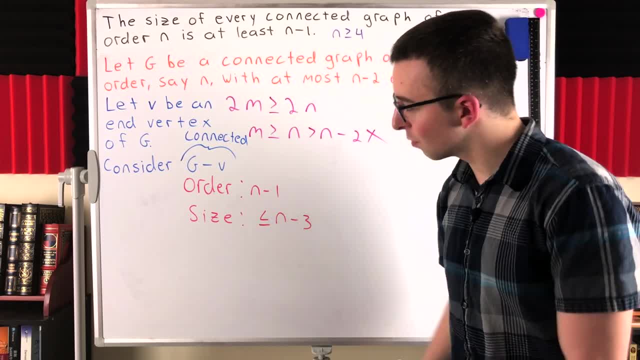 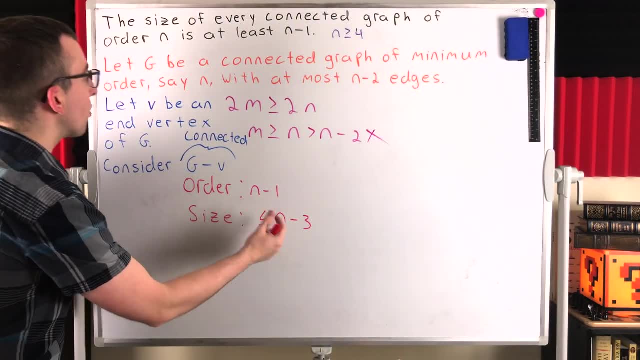 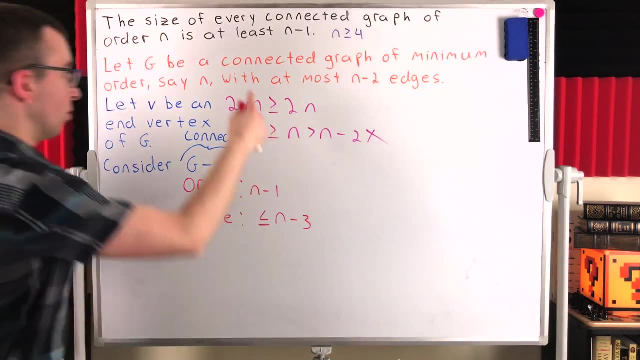 at most two fewer edges than it has vertices. So g minus v is a counterexample and in particular g minus v is a counterexample with fewer vertices than what we assumed was our counterexample of minimum order. That's a contradiction If g is a counterexample of minimum order. 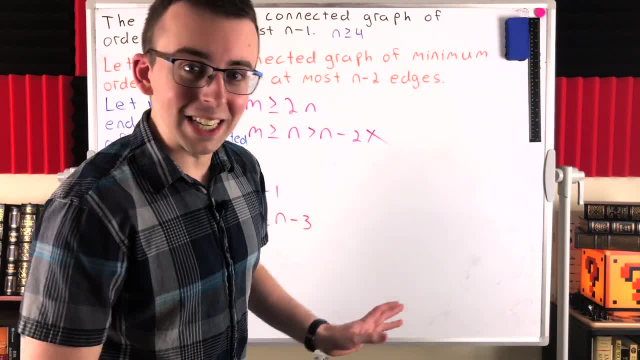 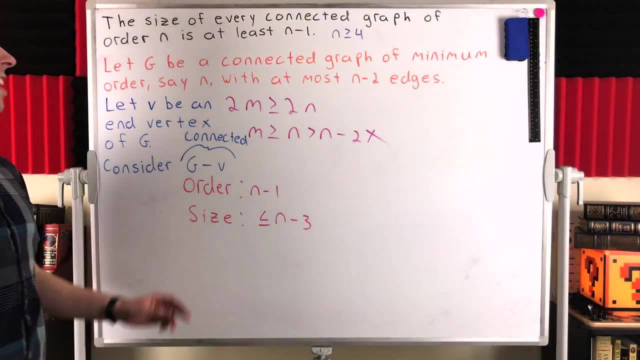 you can't find what was at most 0!. All this kid has to be equal to n-1-0!, a counterexample that has a lesser order. but we did. that's a contradiction. so it turns out there cannot exist any counterexamples at all, and our claim holds The size of every. 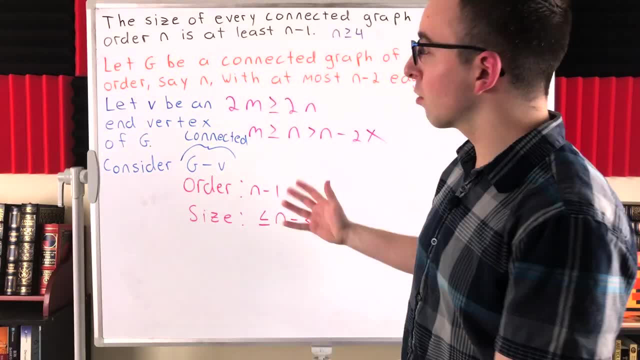 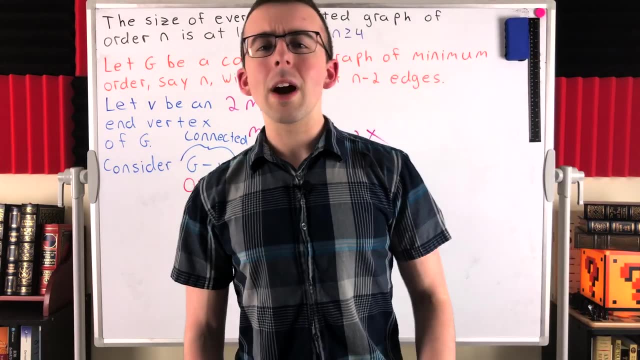 connected graph of order n is at least n-1.. I think it's a really cool result, So I hope this video helped you understand the proof. Let me know in the comments if you have any questions, need anything clarified or have any other video requests. Thank you.